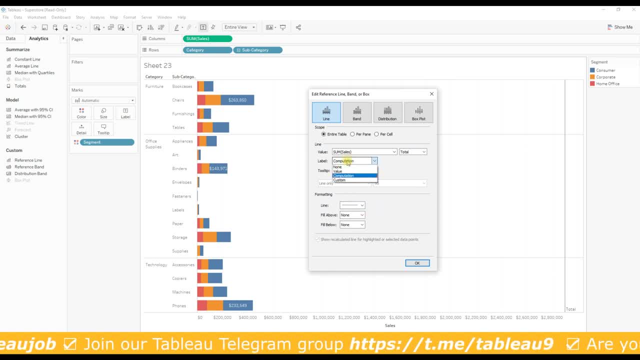 click on this competition. You can click on the label, drop down and select value. If you want to display the value, Okay. so if you want to display the totals per pane- in this case, per pane means per each category, That is, furniture, office supplies and technology- 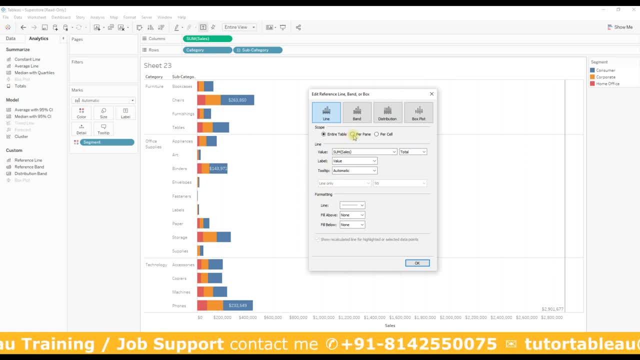 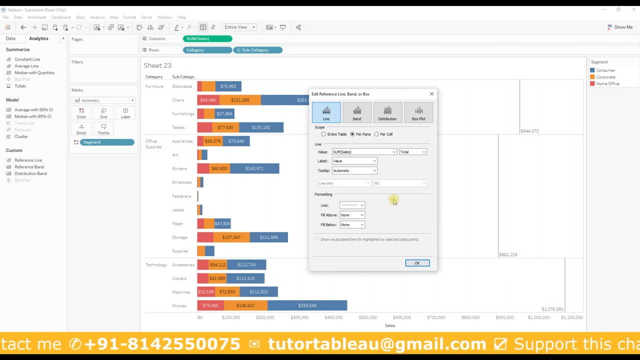 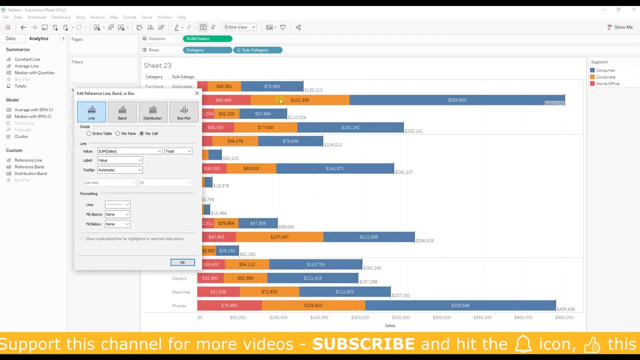 grand totals for each category. you can select per pane. see now, we have the totals displayed per each category. so if your requirement is to show the totals per each bar, that is, per each cell in this view, then you can select per cell. that's it here. we have the totals displayed at the end of each stack bar. 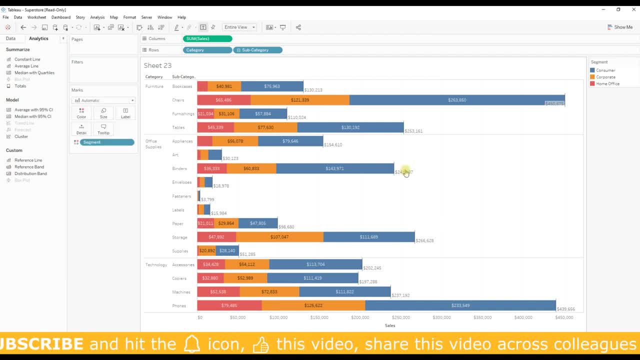 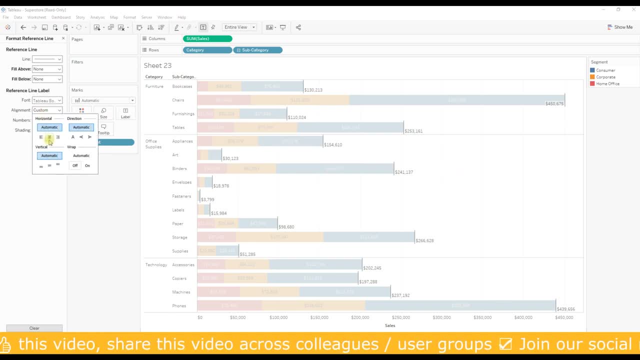 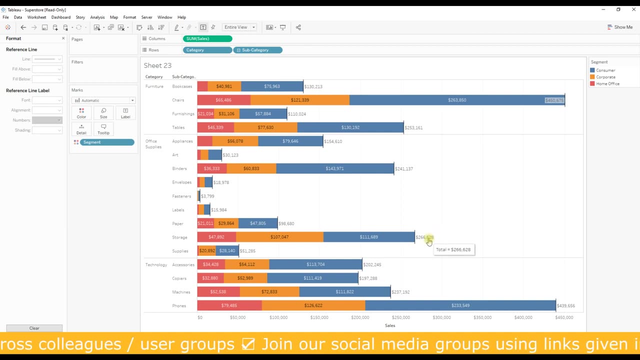 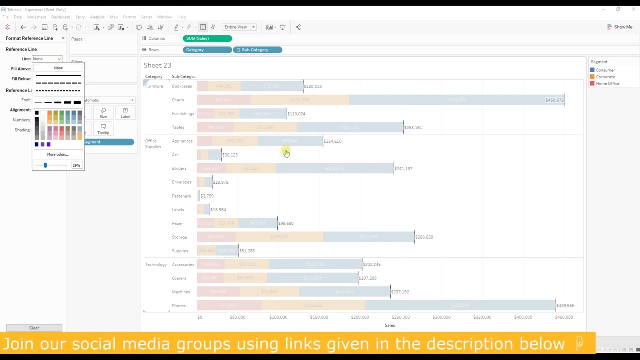 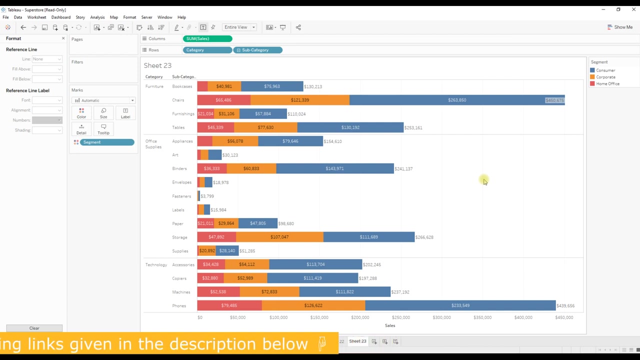 click OK to format these values. you can click on this value and select format, and then I am going to change the alignment to Center. okay, so you can also remove this line. select none: okay, so it's now clearly looks like a totals displayed at the end of each stack bar. I hope this tutorial is. 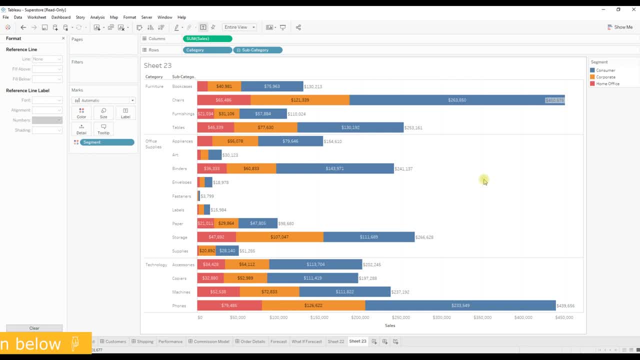 helpful to you. if you like this video, please hit the like button and do subscribe to my channel. thank you for watching. 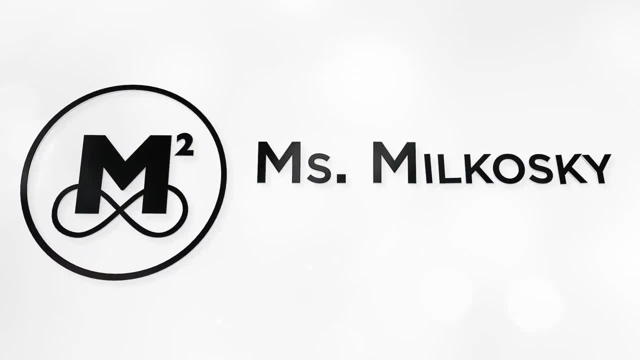 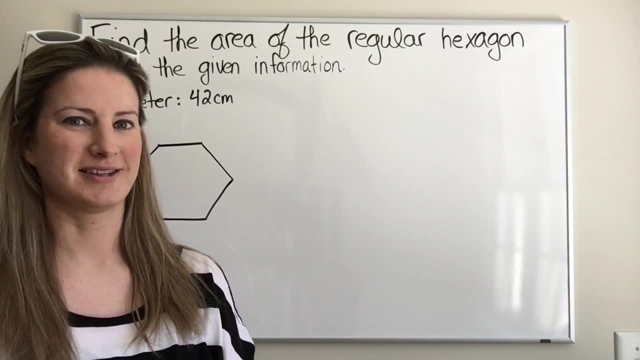 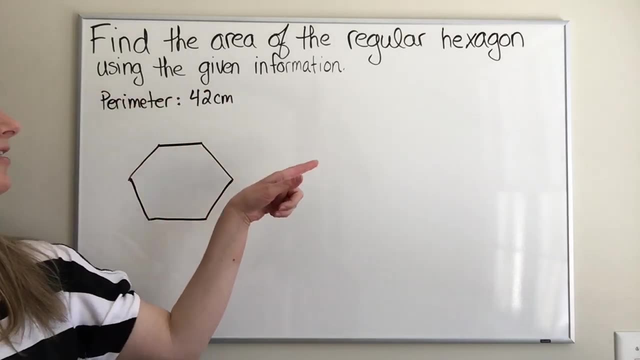 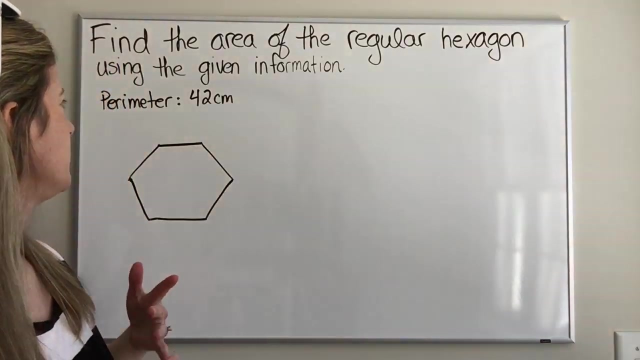 Let's try to find the area of regular polygons. So take a look at this problem right here. So we want to find the area of the regular hexagon using the given information. Okay, So the given information could be the perimeter, it could be a side length, it could be a radius. 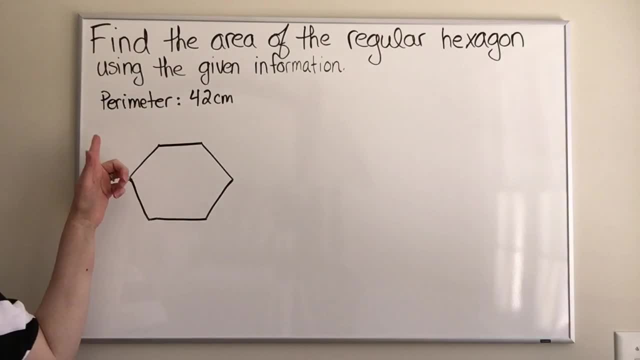 it could be an apothem, any of those things. Okay, So in this case we got the perimeter, So we have to do a little bit of work to start. Okay So, because it's a regular hexagon, we know that all the sides have the same measure. So if the perimeter is 42, a hexagon has six.